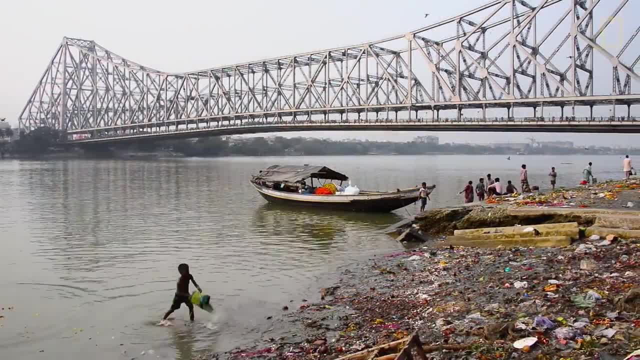 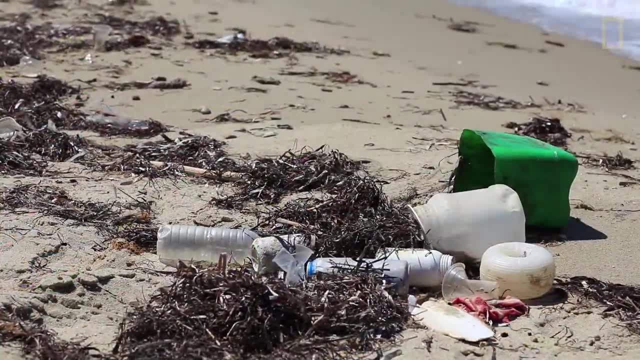 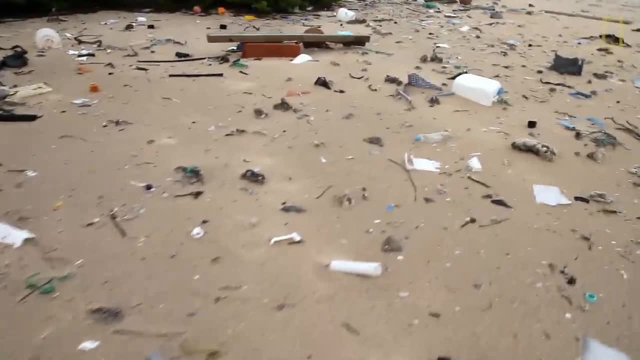 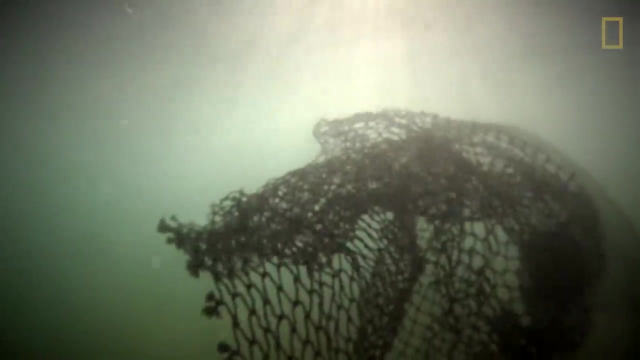 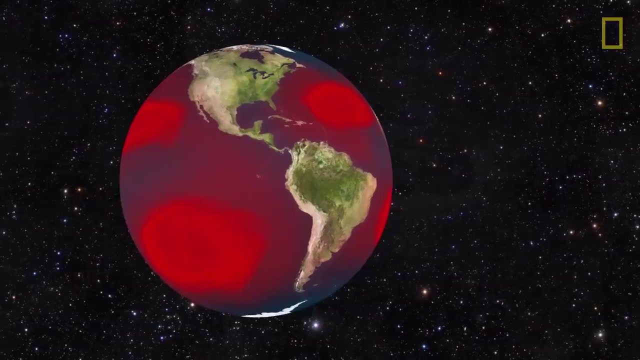 8 million metric tons of plastic trash enters the sea from land every year, The equivalent of five plastic bags filled with trash for every foot of coastline in the world. Across our ocean, plastic trash flows into circulation, Dispersed almost everywhere, but concentrating in huge swaths in the midst of global currents breaking down into smaller. 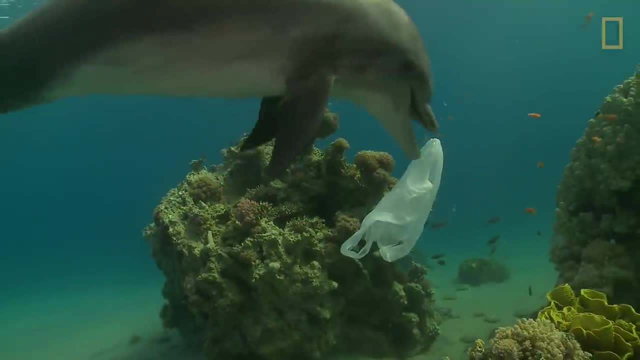 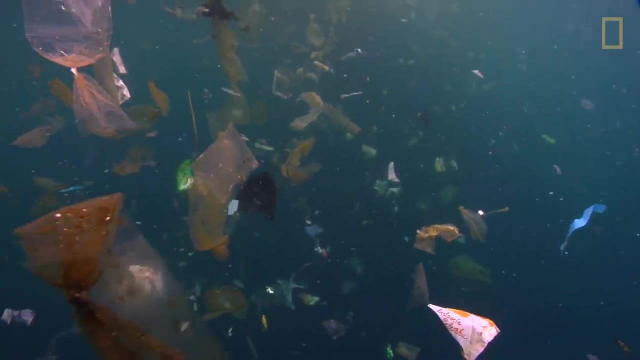 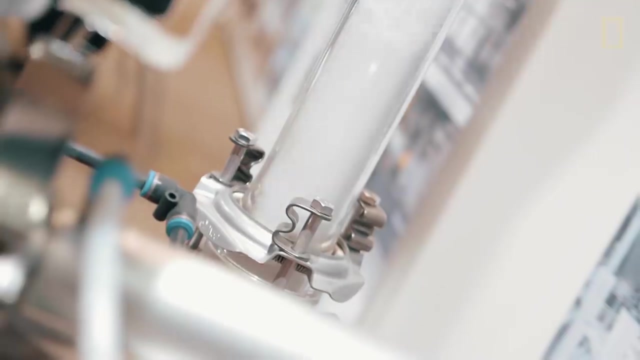 and smaller pieces ingested by species across the marine world and sinking to the bottom of the sea. Anyone can make plastic anywhere in the world and sell it anywhere else in the world. There's no design paradigm, there's no barriers In order to solve the plastic packaging problem. 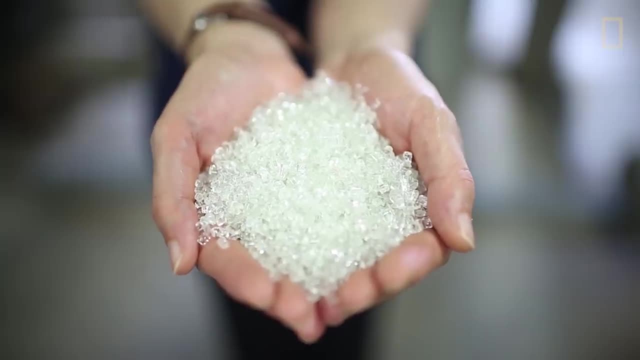 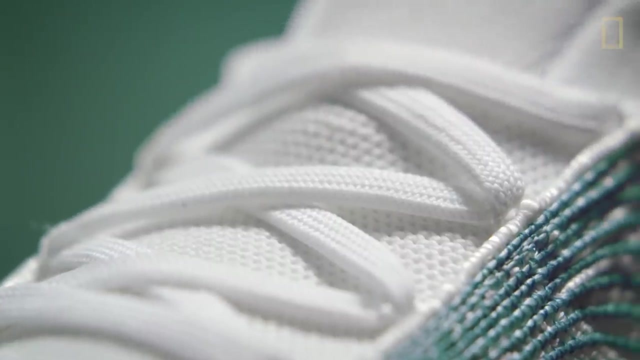 we need to effectively rethink the world From one which is linear- ie take make dispose- to one where it can be recovered and fed back into the economy as a valuable plastic material, or one where it is bio-benign. 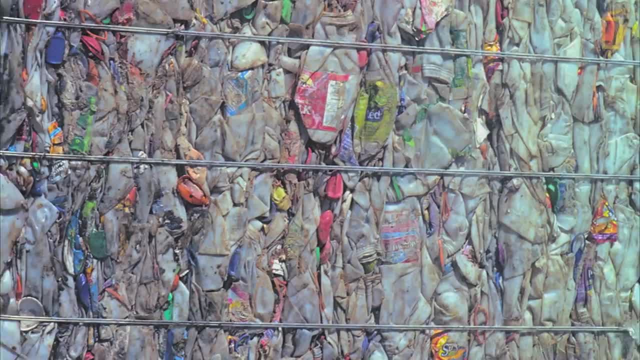 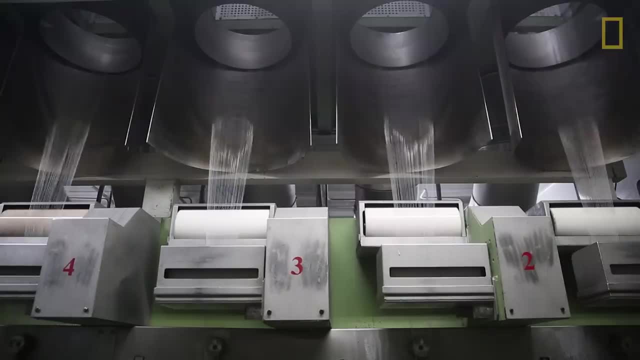 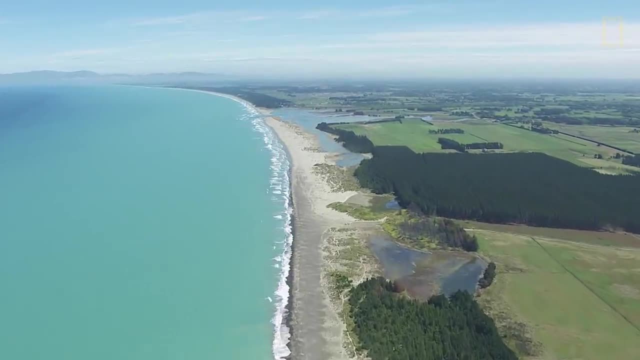 and it can enter the environment. The ultimate goal of the new plastics economy is to design an economy where plastic packaging never becomes waste, And to do that we need every single player in the chain to change the way that they do things. But marine pollution comes in many forms. 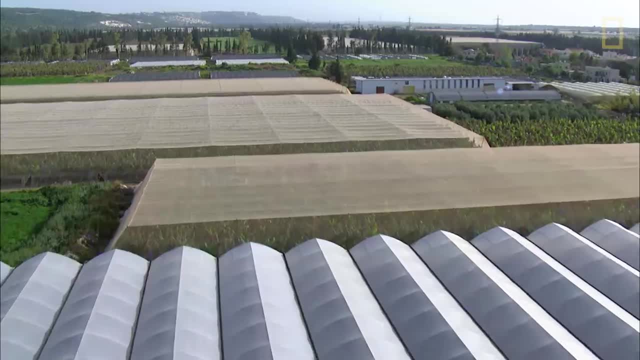 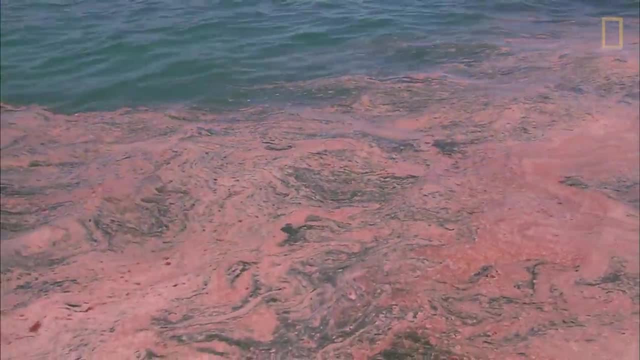 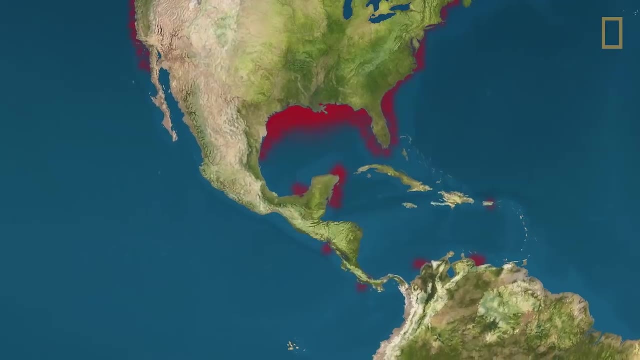 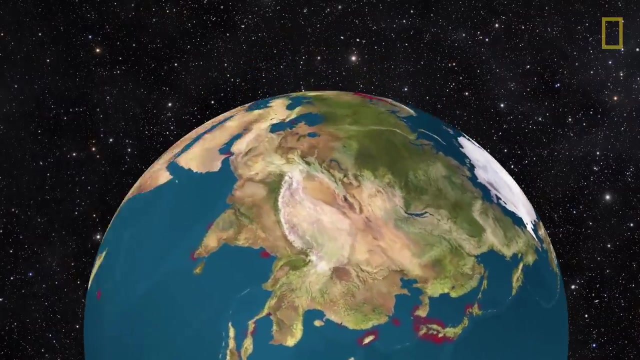 Industrial, agricultural and urban waste also sweep into the sea, fueling explosions of algae that rob marine ecosystems of the oxygen they need to survive. With sustained pollution, these areas become dead zones, which already exist in more than 400 locations across the globe, But nutrient pollution can change the world. 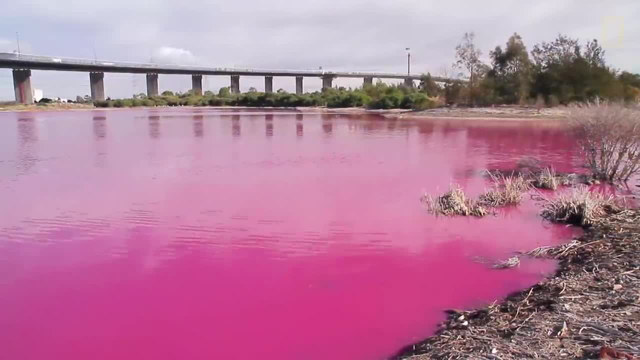 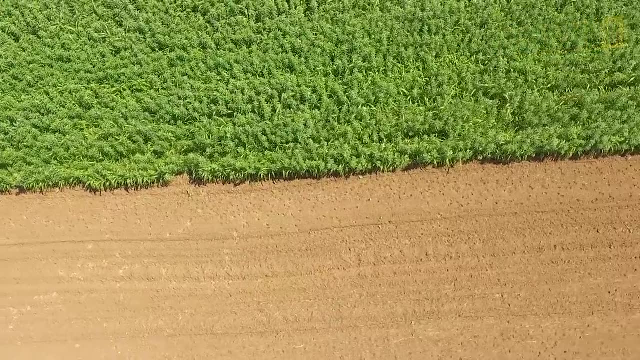 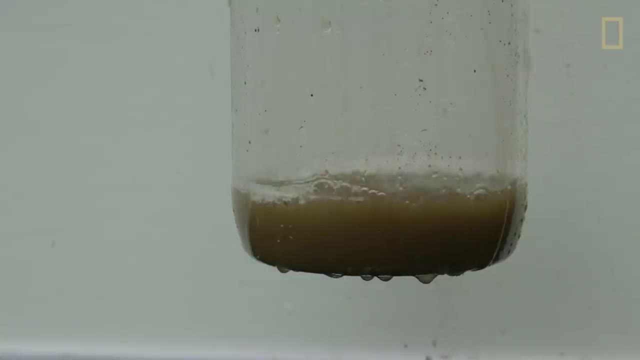 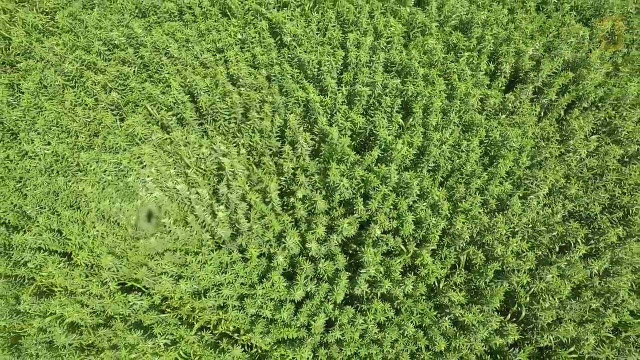 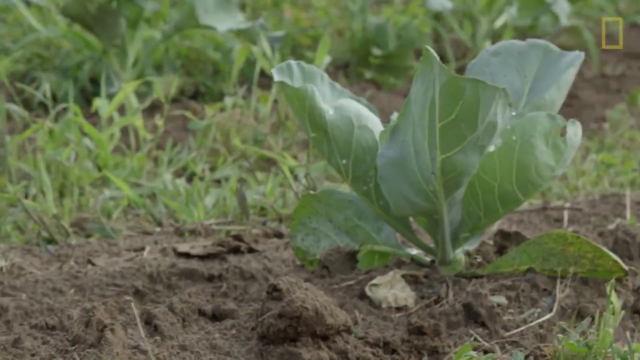 solve. Soil health is critical for water quality. It's the first thing we have to focus on Here on the farm. organic matter is the key thing that we try to improve. The more organic matter you have in the soil, the better the soil can hold on to nutrients like phosphors and nitrogen. Organic 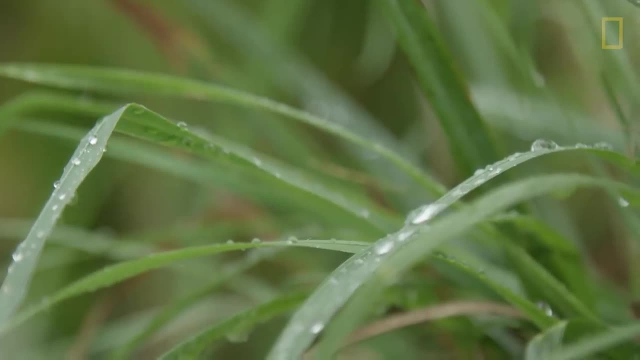 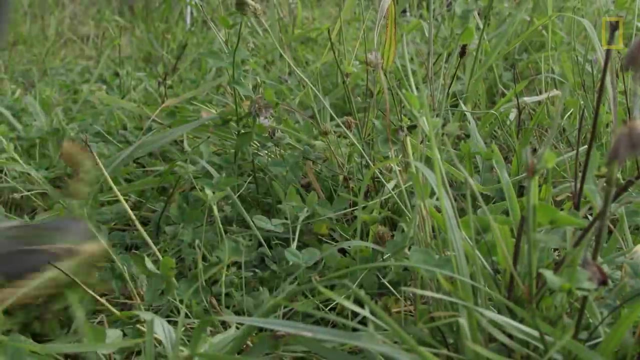 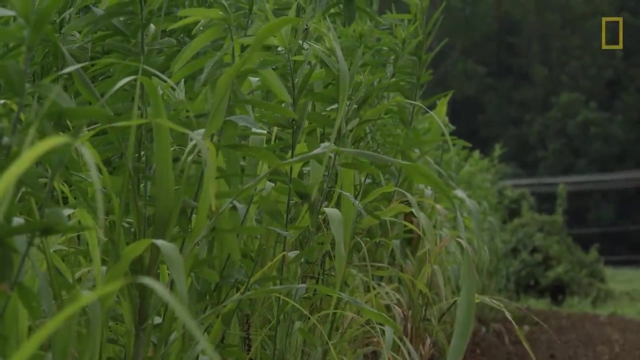 matter keeps it from leaching out of the soil. It grabs onto it and that's good for the farmer, but it's also good for water quality in the bay. For any farmer to change their system is tricky and it takes a lot of work. I think all farmers want to. It's learning different processes. 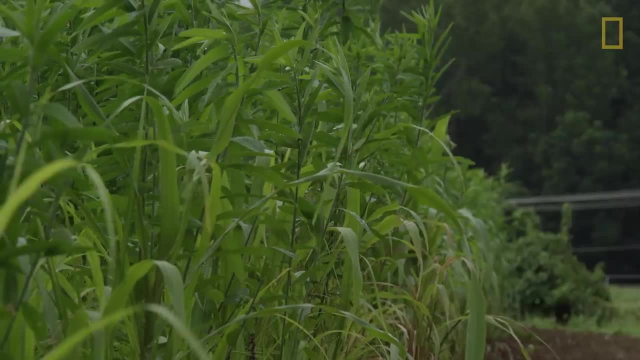 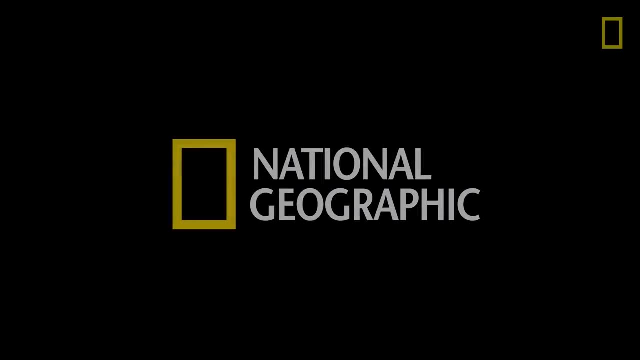 practices that allow you to do it effectively, That becomes a key. 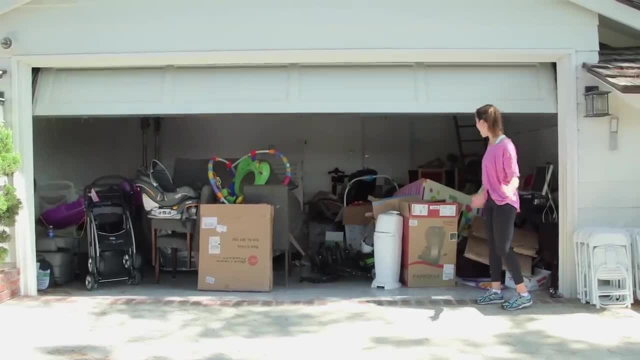 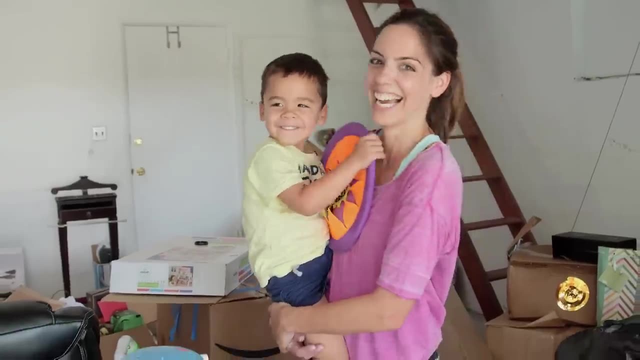 Hey guys, so my garage has gotten a little bit out of control. That is an understatement. I don't know how this happened, but it happened. We definitely have too much stuff, So this week I'm going to show you how I got rid of a ton of it and exactly where I took everything in. 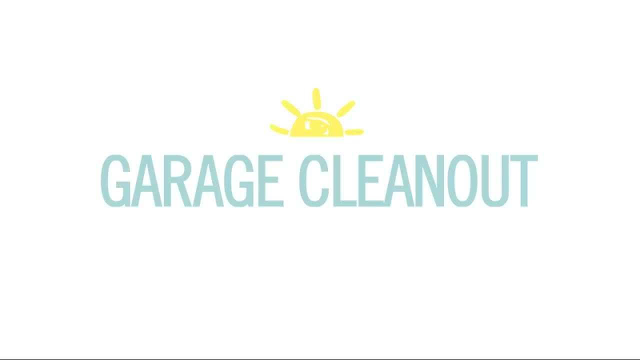 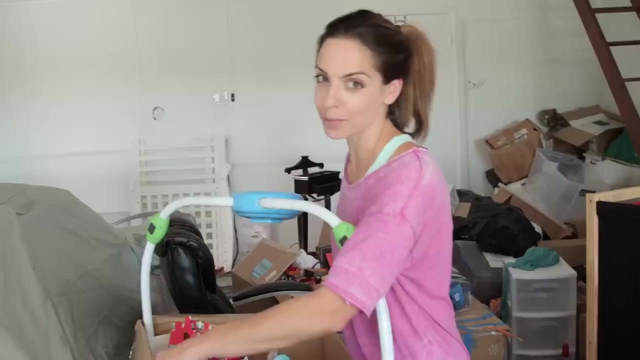 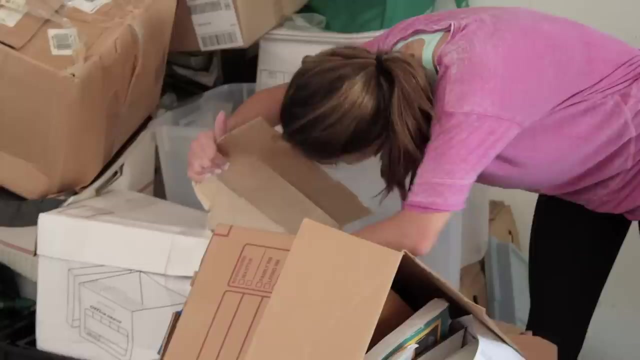 this major garage clean out. So first I had to assess all of the stuff. I'm trying to forge a path: Baby item: We're done with the baby stuff. Stop. We have to keep this for something, I mean, you guys? does Ross really need his college papers? Ah, spider, Oh hi, I don't even want. 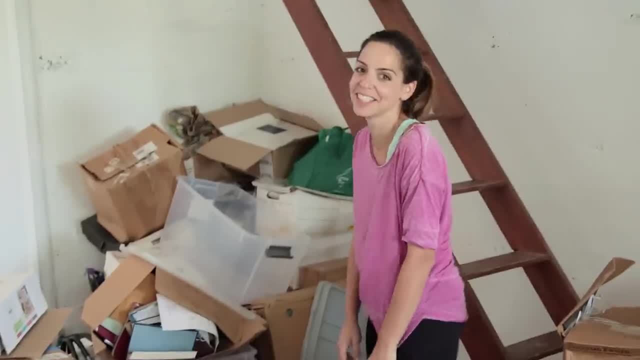 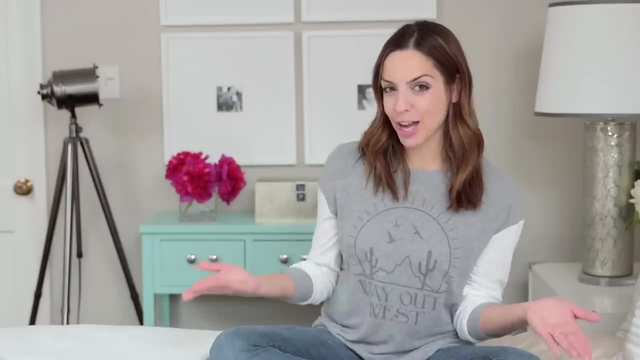 to know what has been spilled on this chair Break. My goal was to either donate or recycle most things, but I still had quite a bit of junk. I thought about calling a junk removal company, but I'm glad that instead I rented a dumpster for three days. 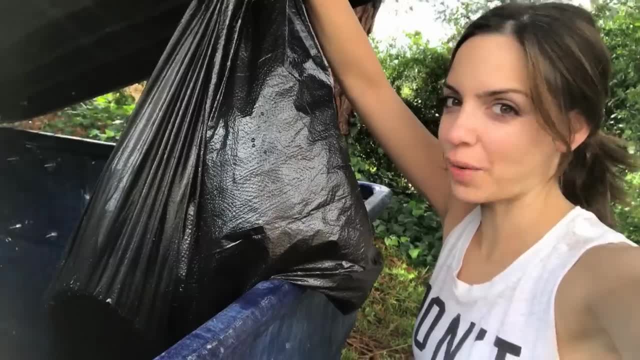 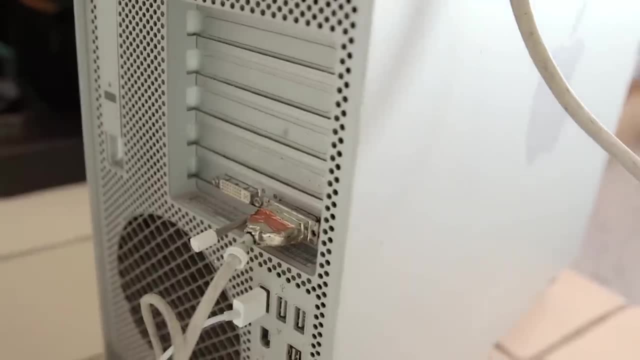 It is so much less money and you can purge less frantically. No hidden labor fees, Just me. Next up, old electronics. Look at these big Mac pros that I spent a lot of time with back in the day. Huge, There was a newer one that was working. I transferred all of the data. I will go through. 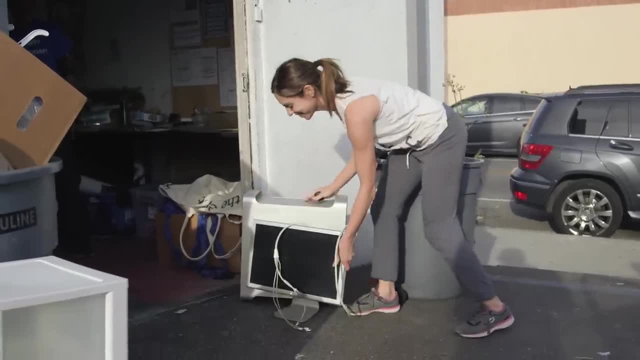 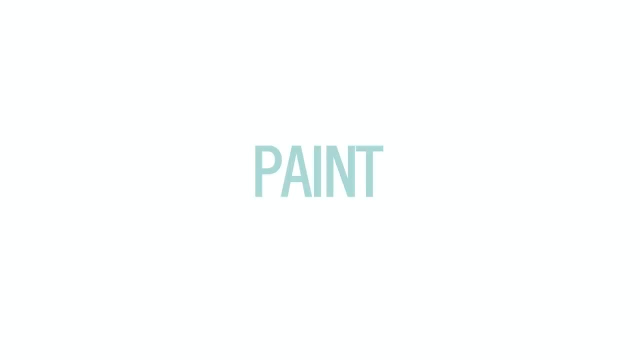